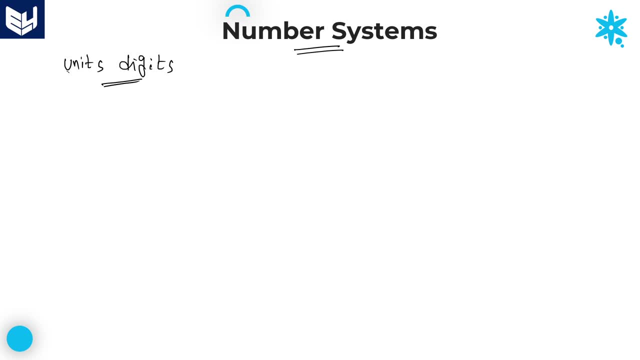 In the last sessions I explained the concept of units digit by using first category digits 0,, 1,, 5, 6 and second category digits 4 and 9.. These two categories are already completed. in the last sessions and also I explained various problems related to these two categories. 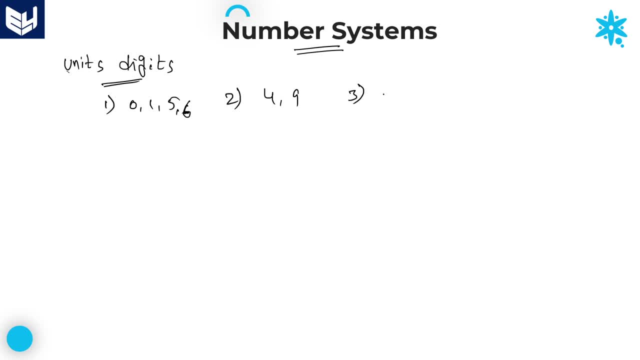 Now in this session I will explain the concept of third category digits, which is 2., 3,, 7, 8.. The concept of third category digits: 2,, 3,, 7, 8.. Once it is done, we will go ahead with problems related to third category digits so that we will finish all the three categories of problems in units placed digit. 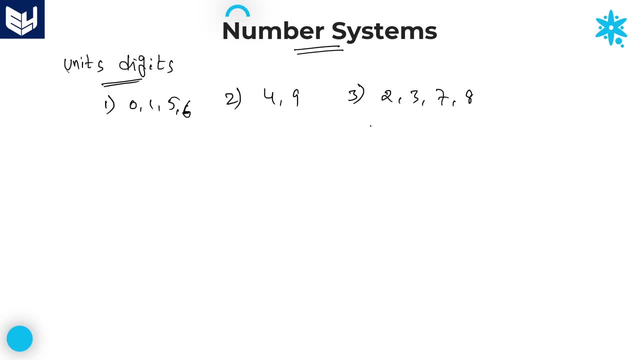 Third category digits also over by this session. In the next session we will discuss the problems based on third category digits. Let me explain the concept first. First, see here: Observe the units places carefully. Here, if any number is ending with 1 and the power values, 2 power 1 is equal to 2, 2 power 2, 4, 2 power 3, 8, 2 power 4, 16, 2 power 5, 32, 2 power 6, 64, 2 power 7, 8.. 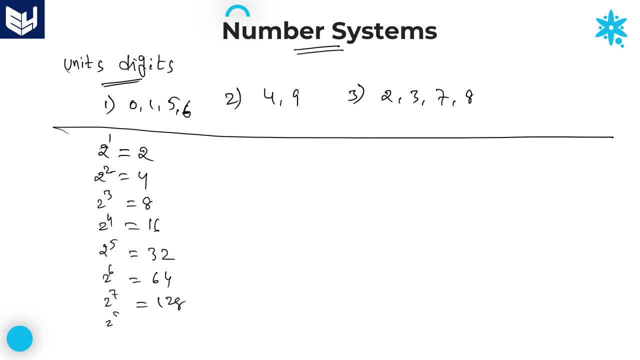 7, 128,, 2 power 8, 256.. If you observe carefully, observe carefully, see here Only 2 power values are very easy to write down up to 2 power 8 or 2 power 10, right. 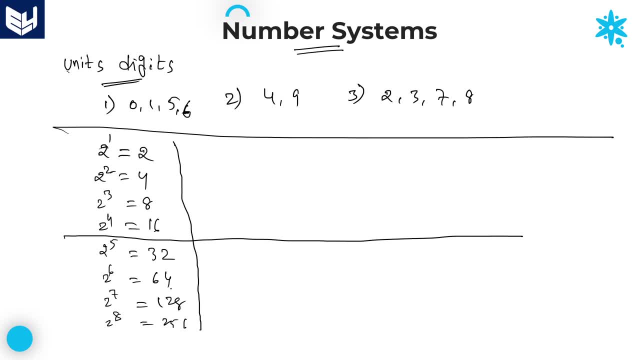 Further numbers. it is not that much of easy task to remember, so that I will write only 2 power values up to 2 power 8, 2 cycles. Observe carefully: For every 4 cycles: 2, 4, 8, 6.. Here the units places are 2, 4, 8, 6.. That is repeated after again 4 cycles: 2,, 4,, 8, 6.. 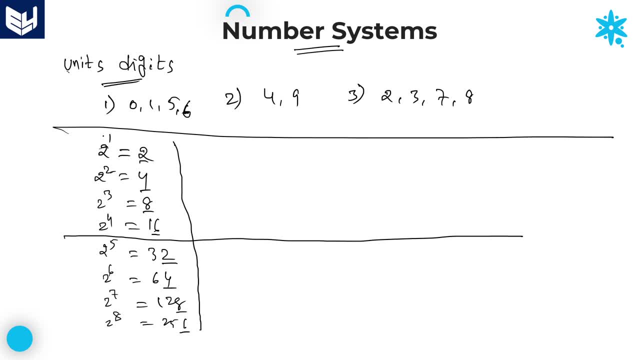 Here the units place digit. In first cycle, first cycle units place and fifth cycle units place. both are same: First cycle and fifth cycle units place values are. both are same Now. therefore the units place is repeated after every 4 cycles. 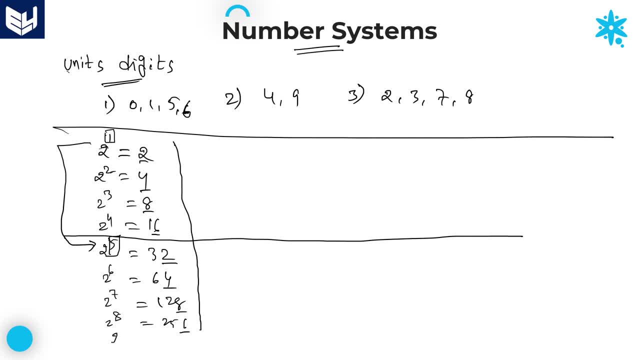 Again, the same units place you will get in the 9th cycle: 2 power 9,, 2 power 9, which is equal to 5, 12.. Again, you will get the same units place in 9th cycle again. 13th cycle. 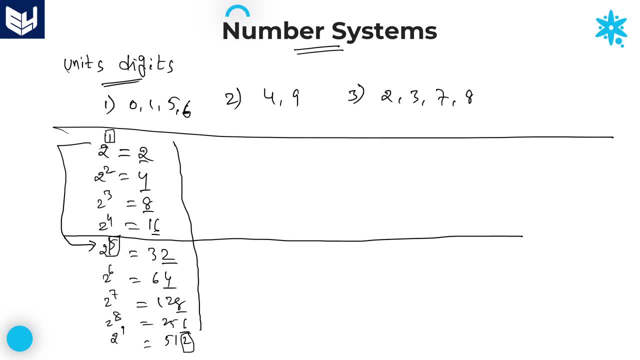 Likewise. it will repeat Similarly for 2. also same thing: 2 power 2 is equal to 4, and it will be repeated after Again: 4 cycles 2 power 6, which is equal to 4 again, and 2 power 3 is equal to 8 and 2 power 7 is equal to 8.. 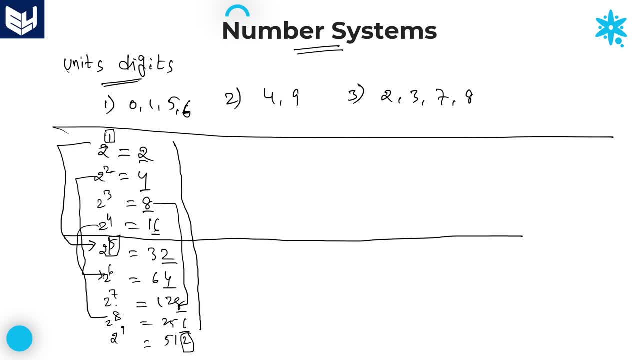 Units place is repeated after every 4, 4 cycles. 2 power 4 is equal to 16 and 2 power 8 is equal to 256. Units place is 6. That is repeated after 4 cycles. So it is very clear that for every 4 cycles the units place values are repeated. 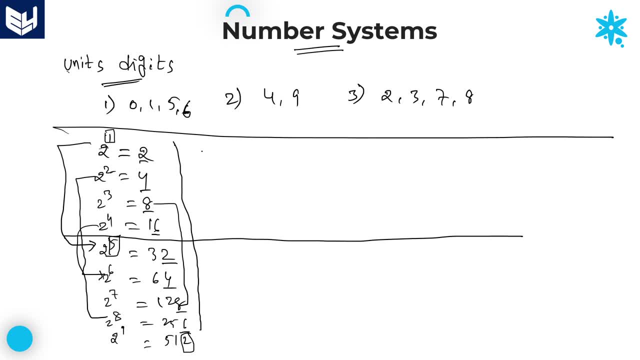 Now we will check it out whether it is applicable for remaining numbers or not. See here: 3 power 1 is equal to 3.. 3 square 9, 3 cube 27.. Here the units place is not repeated anywhere. 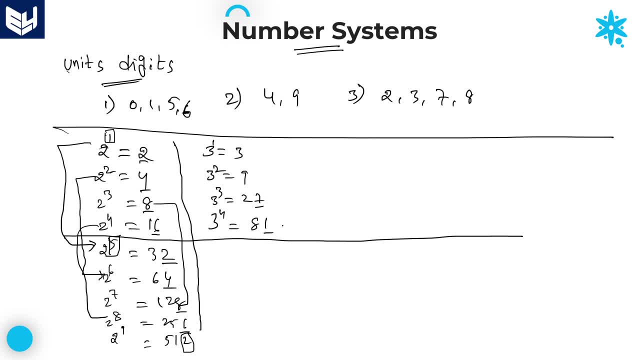 3 power 4,. 3 power 4, 81.. Units place still not yet repeated. 3 power 5,. if you take 3 power 5,, that is 243.. 3 power 5,, that is 243.. 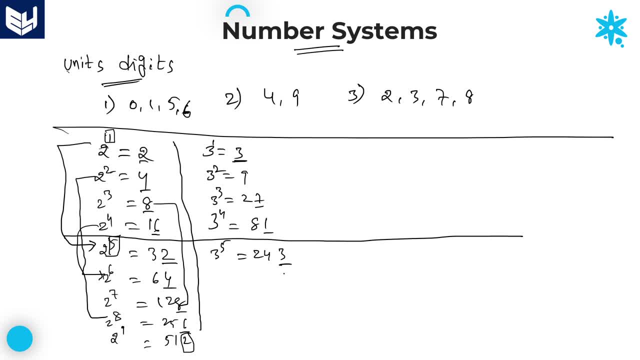 Units place is repeated. Units place is repeated Again the same cycle of 3, 9, 7, 1.. 3, 9, 7, 1.. This cycle will repeat after every 4, 4 cycles. 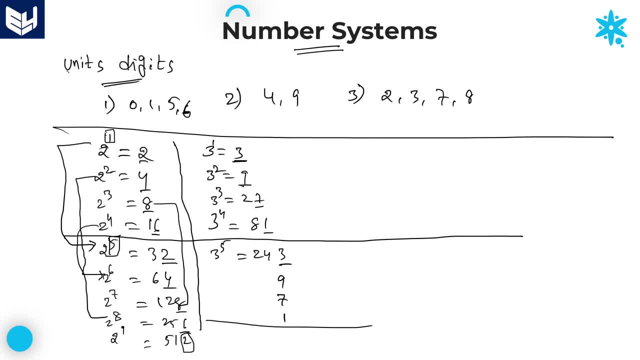 3, 9, 7, 1.. 3,, 9,, 7,, 1.. It means if any number is ending with 3 and the power value. whatever the power value, the possible units places are either 3,, 9,, 7.. 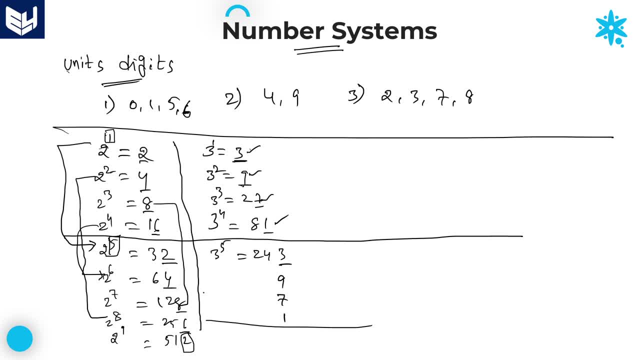 Or else 1.. Only these are the 4 possible units place values. Okay, Now let me check it out for remaining numbers: 7 and 8.. 7 power 1, 7.. 7 square 49.. 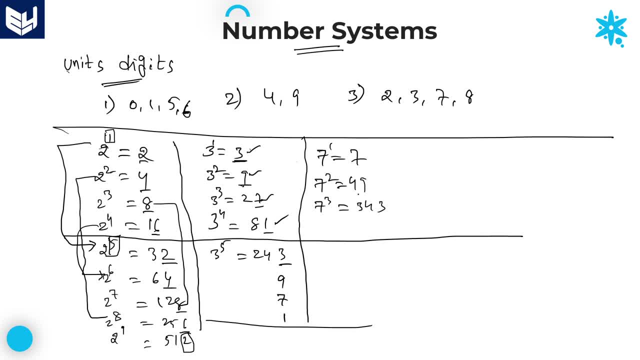 7 cube 343.. Units place: not yet repeated anywhere, Right 7 power 4.. 7 power 4 is equal to 2401.. Even if you don't know that value, it is not a. it is not a big task. 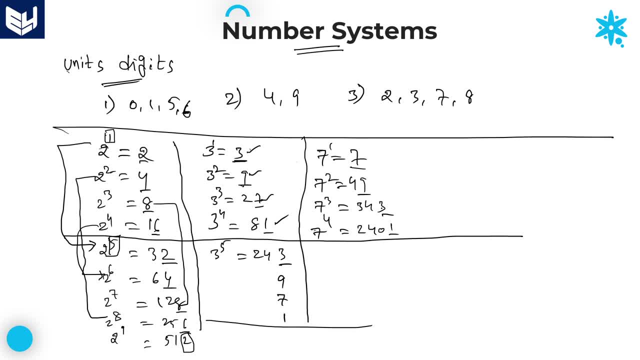 So you just take it out only the units place 3 into 7, 21 units place is 1.. And next I will write here onwards: units places 1 into 7, units place 7.. That is repeated again after 4 cycles. 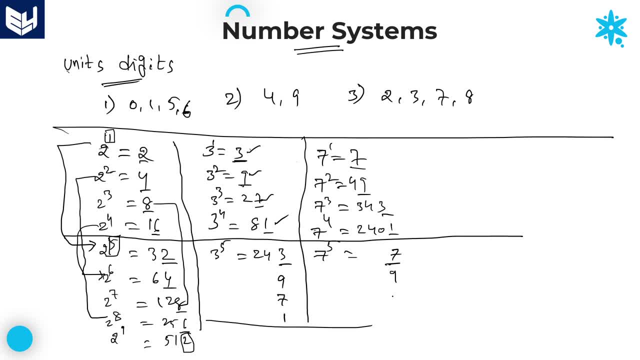 Units place 7.. Right Again, the same cycle of 7,, 9,, 3,, 1.. It will repeat after every 4,, 4 cycles. It means that if any number is ending with 7, and whatever the power value, 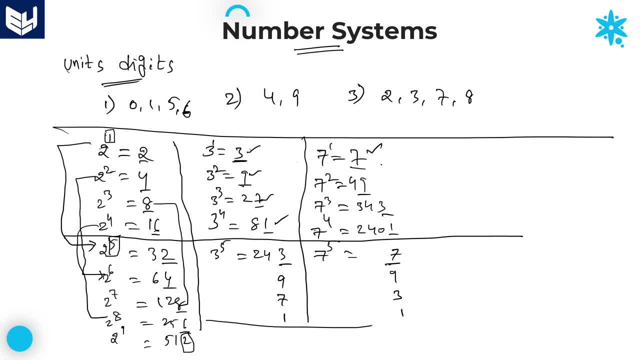 the possible remain the possible units. place values are 7,, 9,, 3, 1.. These are the possible units places. Similarly for 8. also same thing: 8 power 1 is equal to 8.. 8 square is equal to 64.. 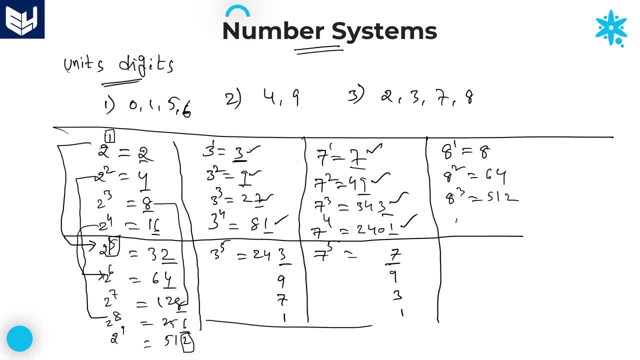 8 cube is equal to 512.. 8 power 4 is equal to units place is 6.. Here it is not mandated to write entire number, So you just write down the units place. Again, 8 power 5 is equal to units place 8.. 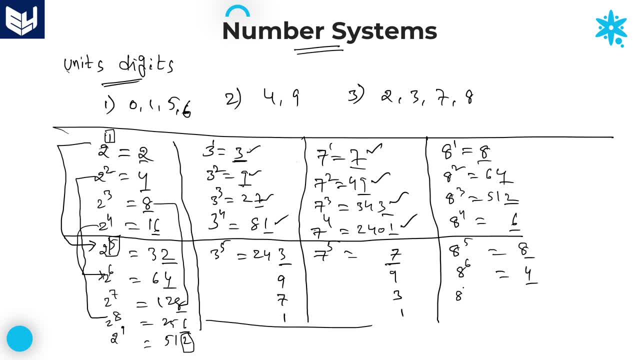 8 power- 6, units place 4.. 8 power- 7, units place is 2.. And 8 power- 8, units place is again 6.. If you observe carefully the units place digit for the number 8,, 8,, 4,, 2,, 1,, 2, 6.. 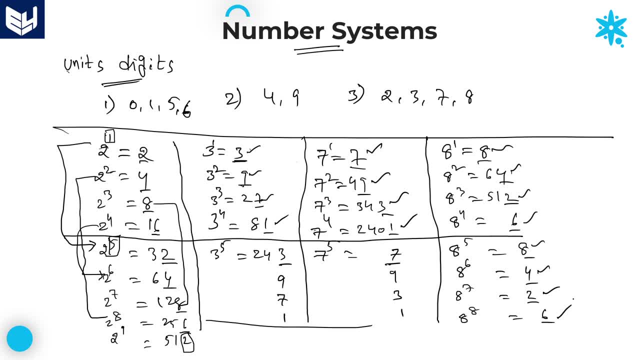 8, 4, 2, 6.. These 4 digits are repeated continuously After every 4 cycles. units, place digits are repeated. Therefore, cycle length of the digits 2, 3, 7, 8,, which is equal to 4.. 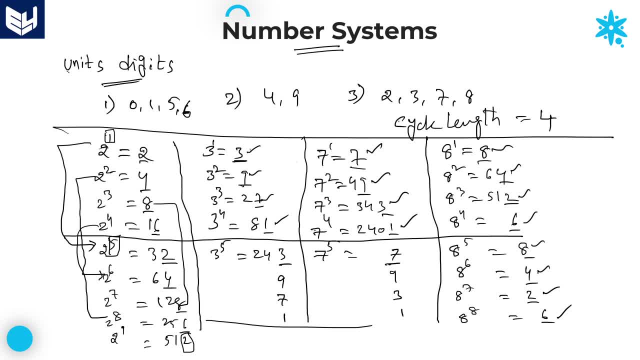 What is meant by cycle length. Do not confuse: After how many cycles units place is repeated, That is called as cycle length, As the name itself suggests. that length of after how many cycles that particular units digit is repeated, Which is called as. 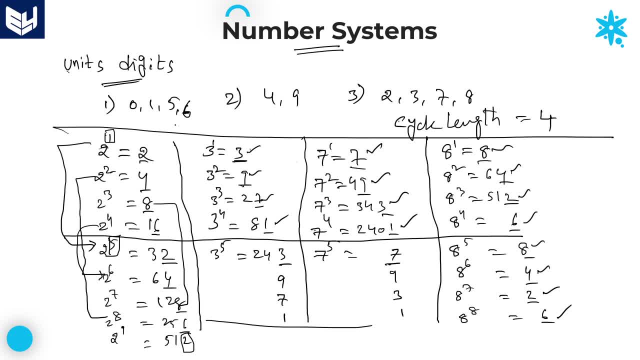 Cycle length For third category digits. For first category and second category digits there is no requirement of doing some calculations. Just by observing the numbers itself we can directly set the answer. But whereas for third category digits there is a small calculation is required. 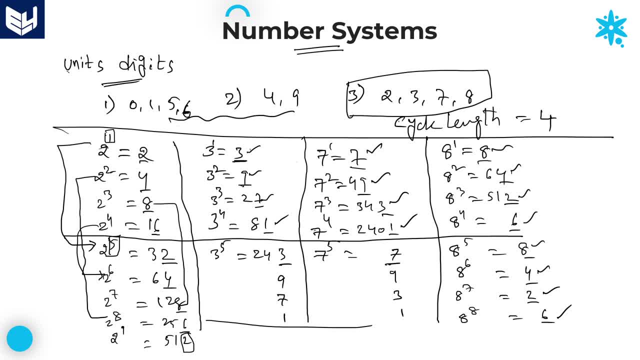 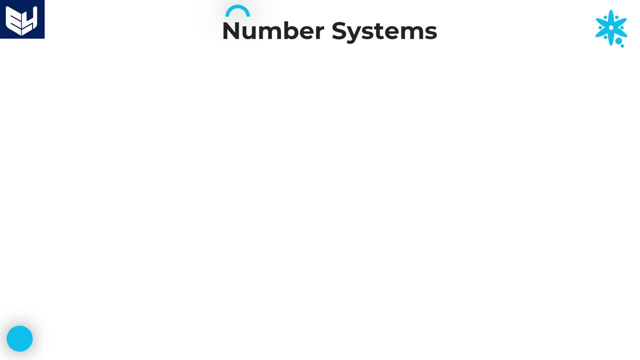 Initially, Initially small calculation is required. Once you are familiar with that, it is very easy to get the units place. Remember the following: The units place value by the second thing and the unit place value. This will be used for any number. 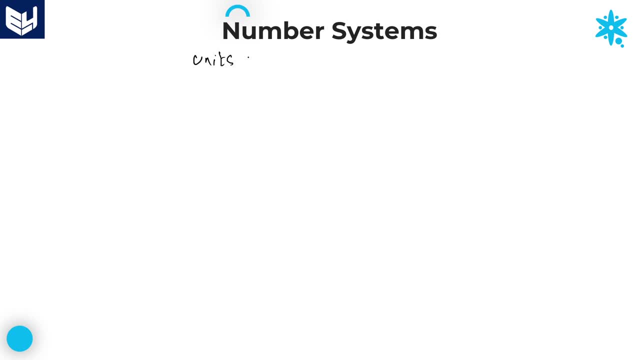 Now your required answers are your required answers If any number is ending with 2.. If any number is ending with 2. Ending with 2., Then the required units: digit is 2 power remainder. Required units: digit is 2 power remainder. 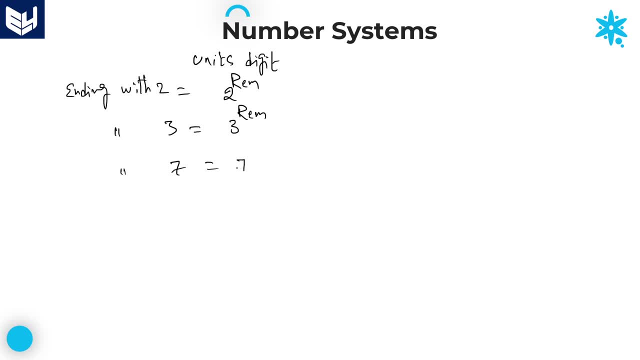 ending with 7, 7 power remainder ending with 8, 8 power remainder. These are your required units place digits. If any number is ending with 2,, then the required units digit is: 2 power remainder ending with 3, 3 power remainder ending with 7, 7 power remainder ending with 8,. 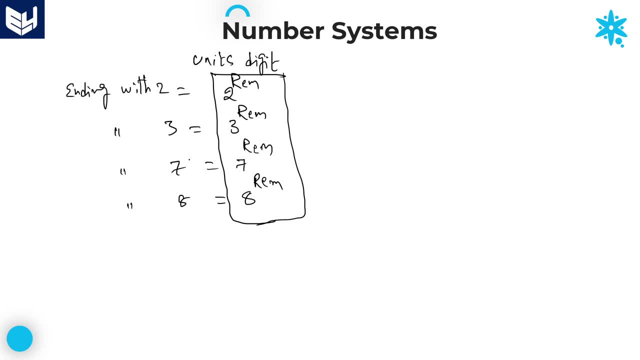 8 power remainder. Therefore now, if you observe carefully how to get the remainder, Once you know what is the remainder value, then it is very easy to set the required units, place digit. right Now I will tell you how to get the remainder. It is very simple: Divide whatever the power value. 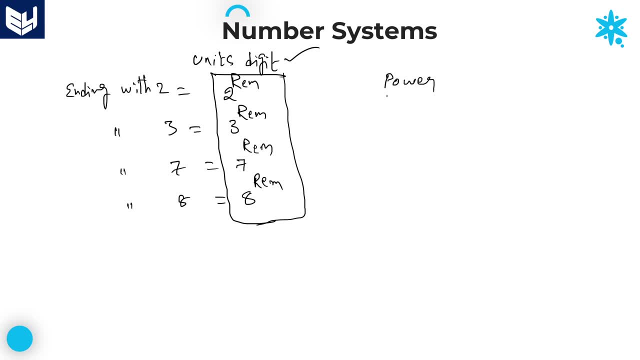 which is given, whatever the power value which is given in the problem, if any number is ending with either 2,, 3,, 7, 8 power remainder, ending with 8, 8 power remainder. Therefore, now, if you 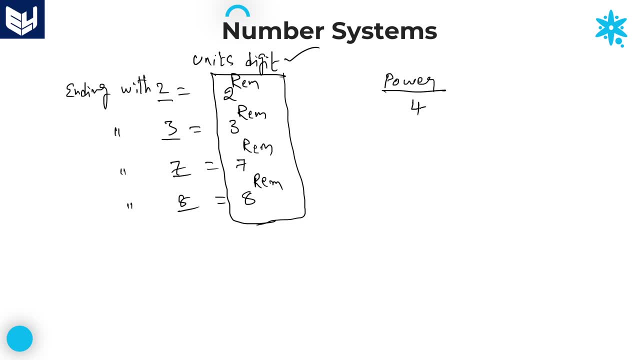 divide the given power value with 4,, this 4 is nothing but cycle length For all the 4 digits. for all these 4 digits- 2,, 3,, 7, 8,- cycle length is 4.. So divide the given power value with 4,. 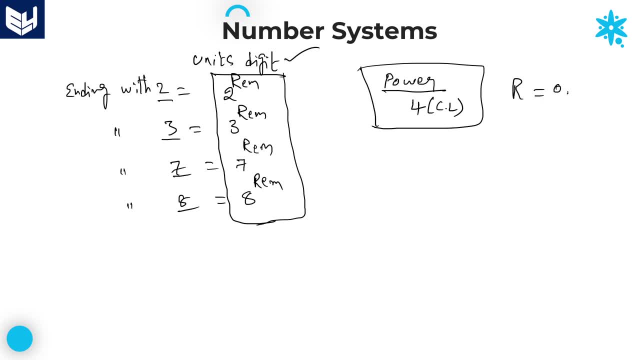 you will get something remainder. You will get something remainder. That remainder value you can substitute over there. Here, your required possible remainders are 0,, 1,, 2, 3.. Why? Because you are dividing the power value with 4. So you will get something remainder. You will get. 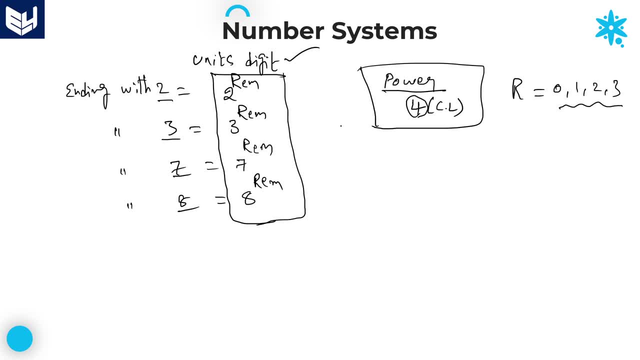 something remainder. When you are dividing any number with 4, your possible remainders are 0,, 1,, 2, 3, only right, You can substitute those values. In this case you will get the required answer. okay, And here let me explain one small example: 2 power 35,, 2 power 35,, 2 power 35. Here. 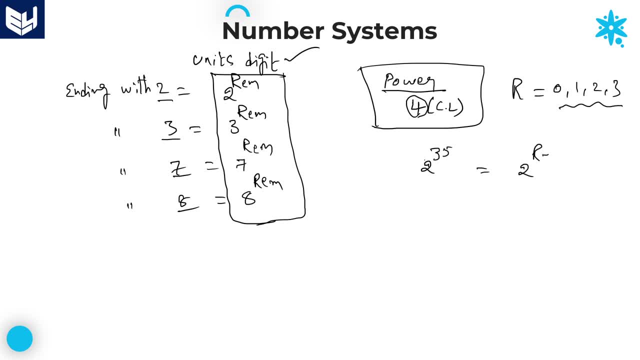 the number is ending with 2.. Therefore, the required units place is 2 power remainder, 2 power remainder. How can you get the remainder here? Divide the given power value: What is the power value? 35 divided by cycle length. 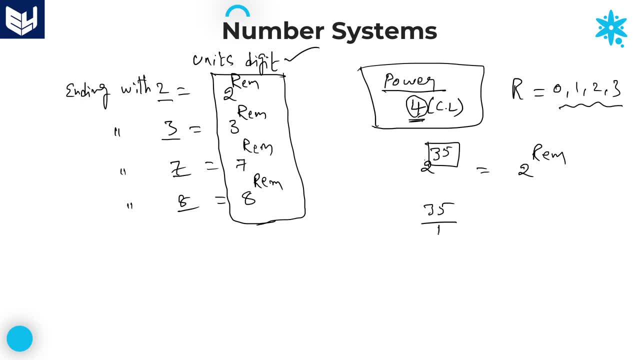 of 2.. What is the cycle length of 2,, which is 4? 35 divided by 4.. Remainder is equal to 3.. Remainder is equal to 3.. Therefore, your required answer is 2 power 3,, which is equal to 8.. 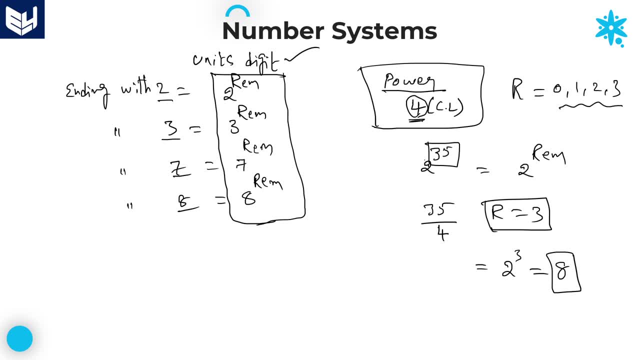 2 power 3, which is equal to 8.. Now, one important point you must be remember is if you are getting remainder 0, if you are getting remainder 0, you should not substitute directly 2 power 0 or 3 power 0,, 7 power 0 and 8 power 0. You should not substitute directly 0.. In place of 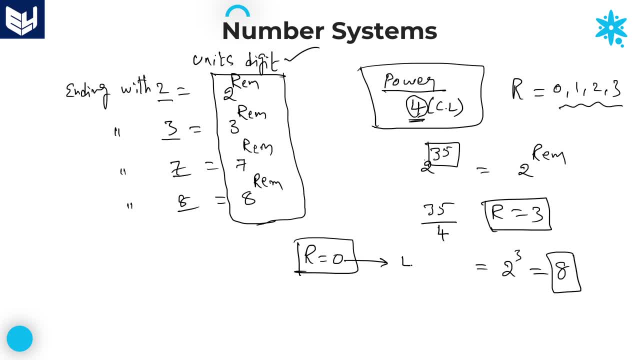 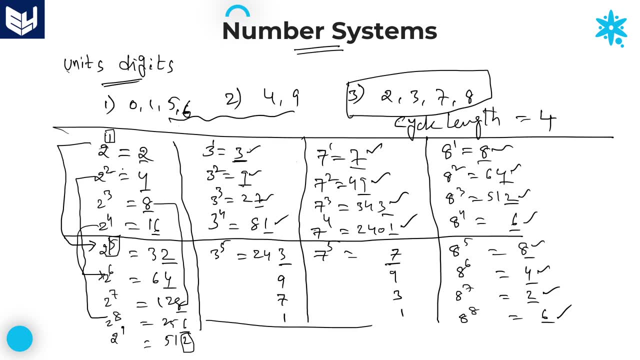 0,. you must be substitute 4.. Why? Because I will tell you In the previous slide. see here: if you are getting a remainder 1, if you are getting a remainder 1, that is in first cycle. That is in first cycle. If you are. 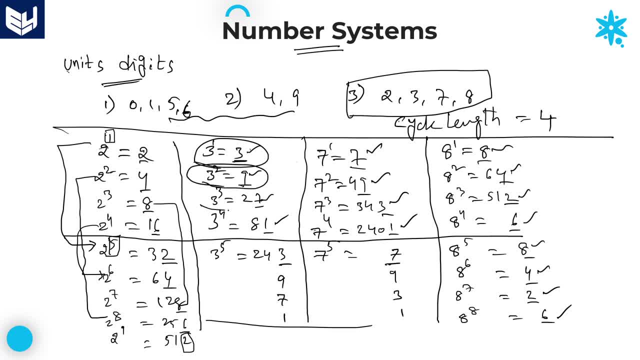 getting remainder 2,, that is in second cycle. If the remainder is 3,, that is in third cycle. But you are not getting the remainder 4 while dividing with 4, right? So whenever you are getting remainder 0, substitute that value to get the remainder 1.. So you are getting the remainder. 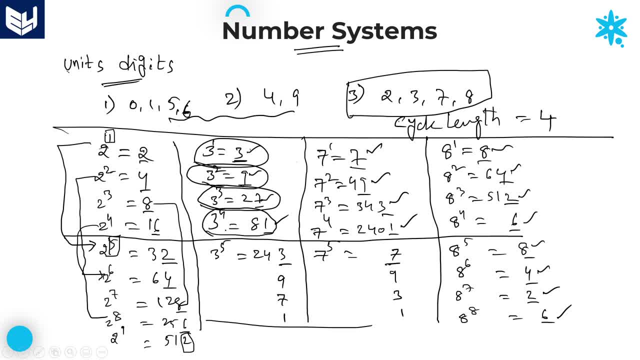 value as 4 instead of 0. that is the only thing you need to remember whenever you are solving the problems related to third category digits. only point you must be remember is whenever you are getting remainder- 0 substitute in place of 0. 4 in place of 0, substitute 4. why? because 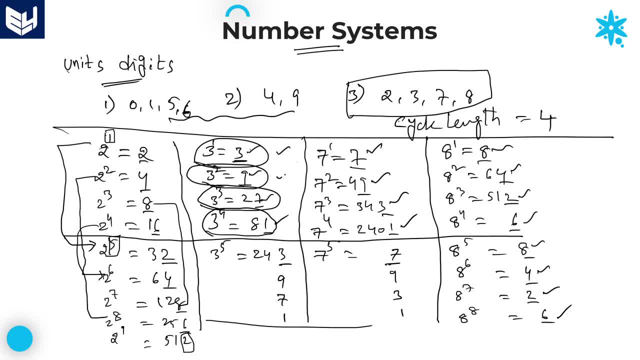 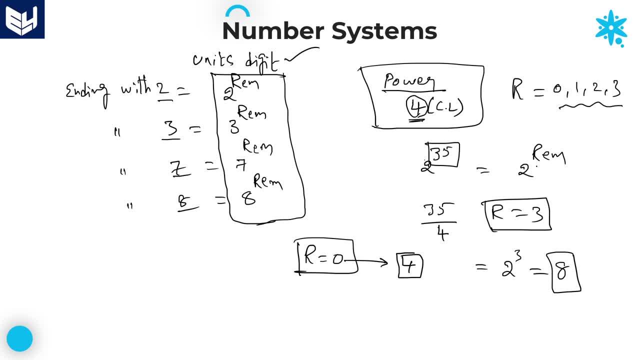 remainder 1 indicates first cycle, 2 indicates second cycle, 3 indicates third cycle. but you will not get remainder 4 while dividing with 4. because of that reason you must substitute. if the remainder is 0, that is in fourth cycle, that is in fourth cycle. so you need to substitute. 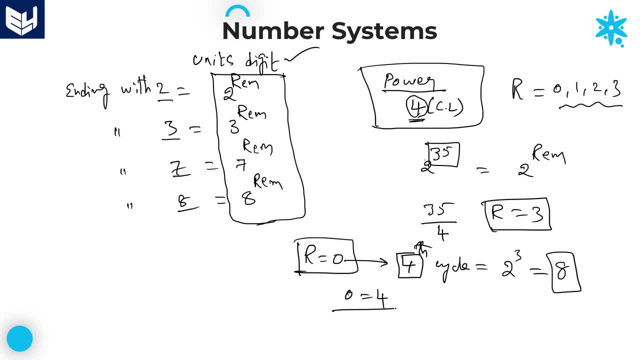 fourth cycle, 0 is equal to 4. whenever you are getting remainder 0, substitute r is equal to 4. that is the only point. you must be aware of that, guys. this is about the concept of a third category: digits, units, place. how to find units, place, digit of any number which is ending. 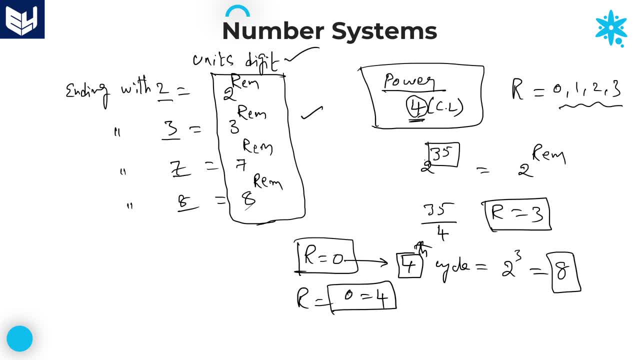 with 2, 3, 7, 8, your required answer is only: 2 power remainder. 3 power remainder. 7 power remainder 8 power remainder. how to get the remainder? just by dividing the given power value with 4 and that not required to divide entire power value. take only last two digits. suppose, for example, if you 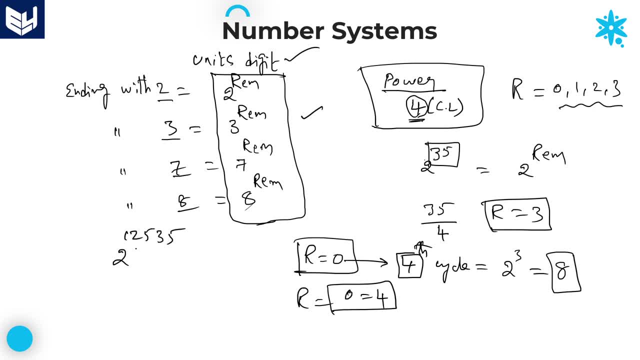 take. this is the number. there is no requirement of dividing entire number with 4, just take only last two digits. the reason is the divisibility rule of 4 is if the last two digits are divisible by 4, then that particular number is divisible by 4. here we divided 35 with 4. you are getting a remainder 3. similarly, when you